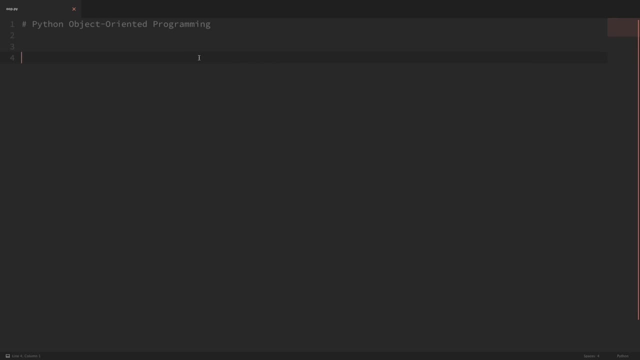 we call those attributes and methods, and you'll hear me use those terms a lot throughout these videos. So when I say methods, I mean a function that is associated with a class. So let's go ahead and get started. So say, we had an application for our company and 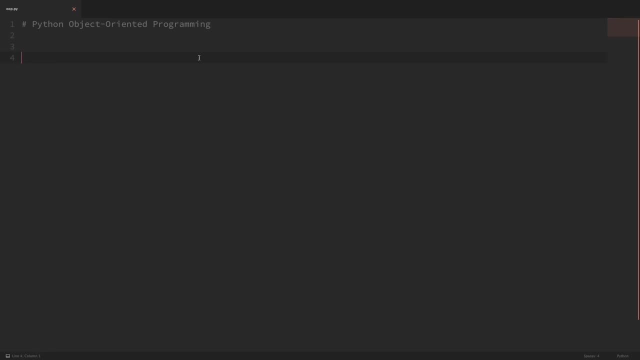 we wanted to represent our employees in our Python code. Now, this would be a great use case for a class, because each individual employee is going to have specific attributes and methods. So, for example, each employee is going to have a name, an email address. 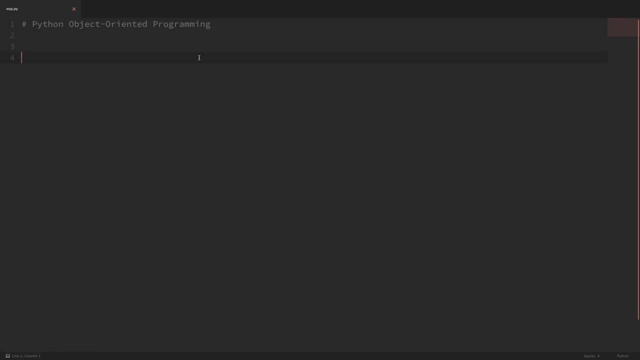 pay and also actions that they can perform. So it'd be nice if we had a class that we could use as a blueprint to create each employee, so that we didn't have to do this manually each time from scratch. So let's go ahead and create a simple employee class and see what that would look like. 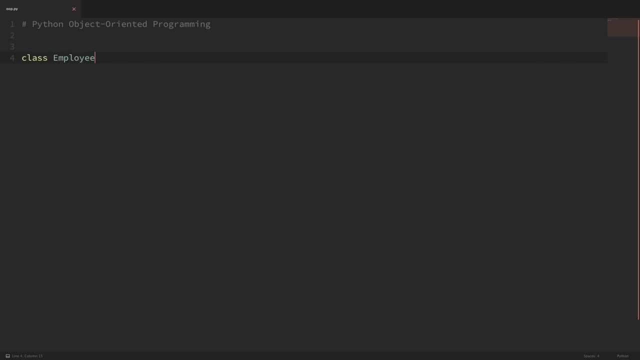 So to create a class, it's just as easy as saying class: employee. Now, I'm going to leave this empty for now, and if we just left it like this, then we'd get an error. So if you ever have a class or a function that you want to leave empty for the time being, you can just go ahead and create a. 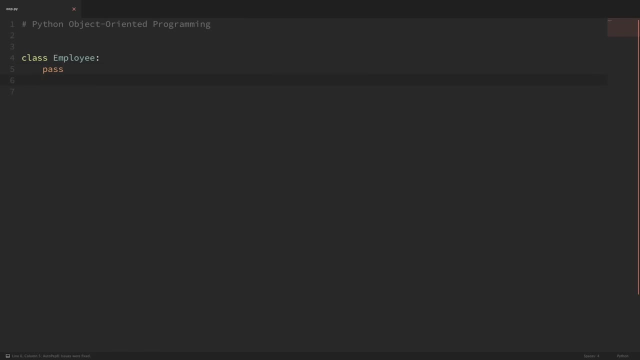 class, Then you can simply put in a pass statement and Python will know that you just want to skip that for now. So now we have a simple employee class with no attributes or methods, And I wanted to stop here because I wanted to explain the difference between a class and an instance of a. 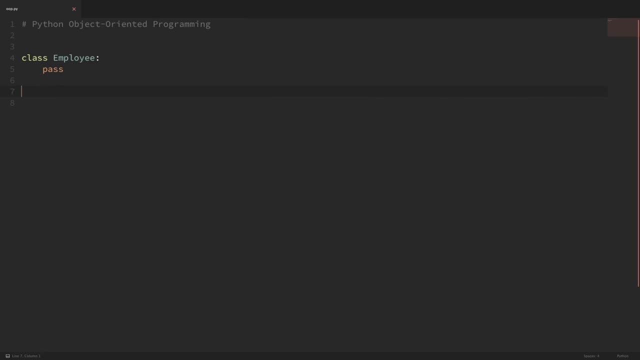 class. So our class is basically a blueprint for creating instances, and each unique employee that we create using our employee class will be an instance of that class. So, for example, if I said one equals employee and employee two equals employee, then each of these are going to be: 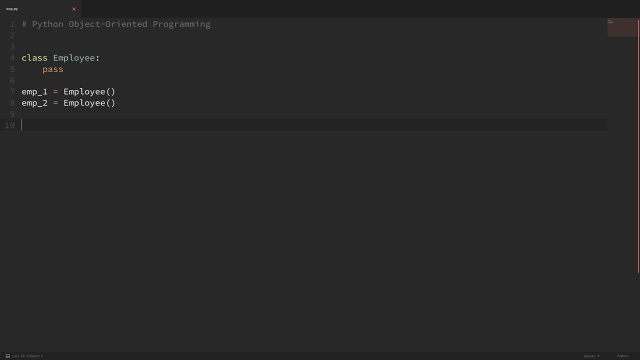 their own unique instances of the employee class. So, for example, if I go ahead and print both of these out and copy and paste that there and you can see that both of these are employee objects and they're both unique, They both have different locations here in memory. Now, this is an important distinction between a class and an instance of a class. So if I go ahead and print both of these out and copy and paste that there and copy and paste that there and you can see that both of these are unique instances of a class. So if I go ahead and print both of these out and 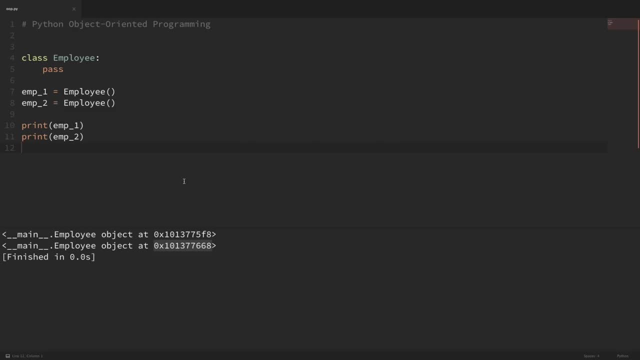 because you'll hear me talk a lot about instance variables and class variables and it's important to know the difference between those, And I'll go more in depth into class variables in the next video, But for this video we're going to be looking at instance variables, So instance variables. 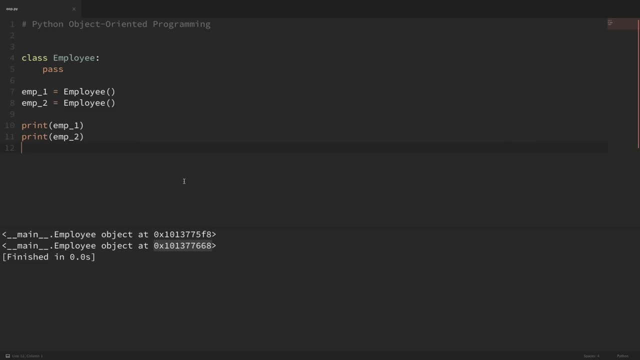 contain data that is unique to each instance. Now we could manually create instance variables for each employee by doing something like this. So let's say we wanted employee one to have a first name and a last name, So I could just do employee one and I could do instance variables for each. 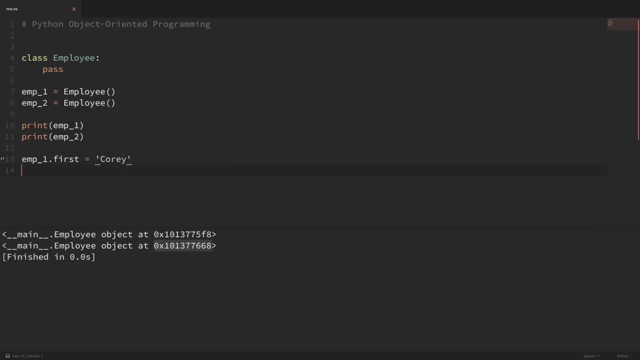 employee, And then I could do: employee last is equal to Schaefer, And I could also give it an email address. So I'll do employee one dot email equals, and I'll just do the first name with the last name at companycom. And lastly, let's go ahead and add a pay onto there too. So I'll do. 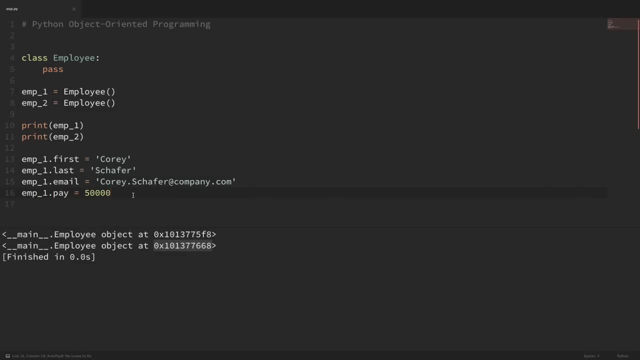 employee one dot pay, and we'll just do employee one dot pay, And then I'll do employee one dot pay. Now let's give employee two some of these same attributes. So for this one I'll just do test user and then I'll do test user and I will make that 60,000.. Okay, so now each of these instances, 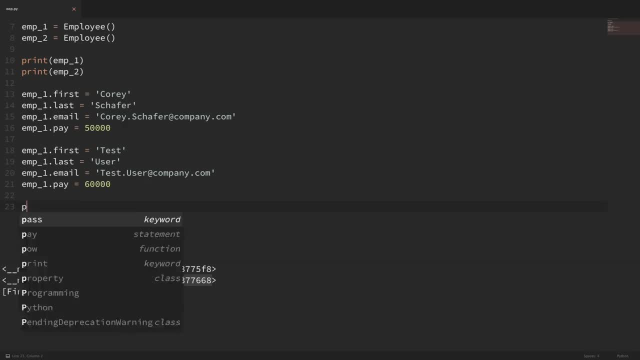 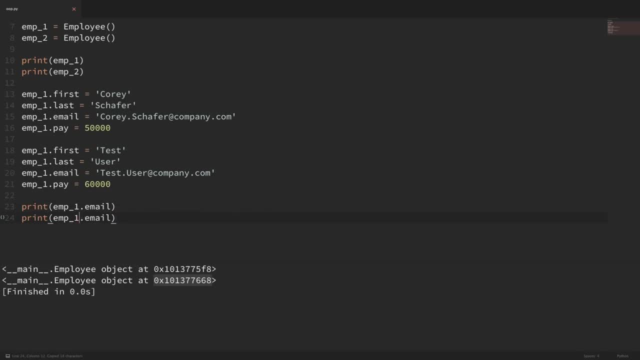 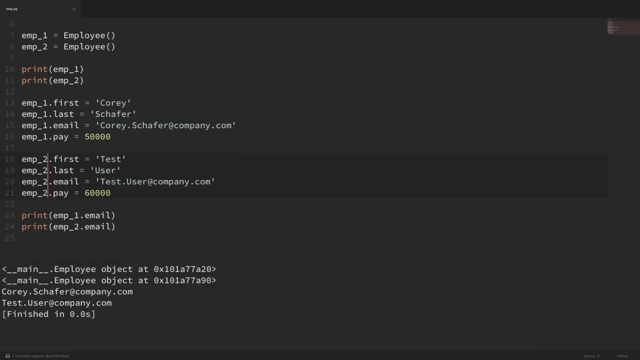 print out the employee two dot email. Oh, and it looks like whenever I gave these the instance variables, I forgot to make this employee two here. So now let's run that. So now you can see that that email was created for each employee. But let's say that we wanted to set all of this. 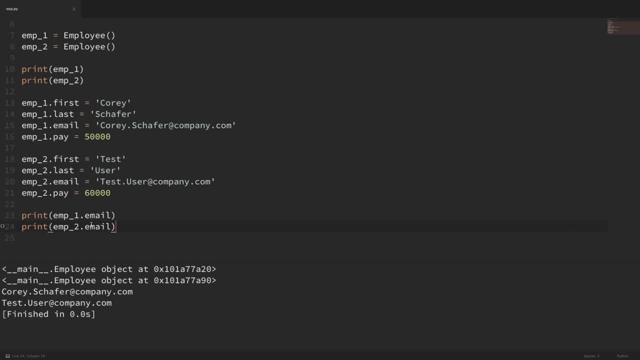 information for each employee when they're created, rather than doing all of this manually like we did here. So we wouldn't want to have to manually set these variables every time. You can see, it's a lot of code and it's not going to be able to set all of these variables manually, So we're going to 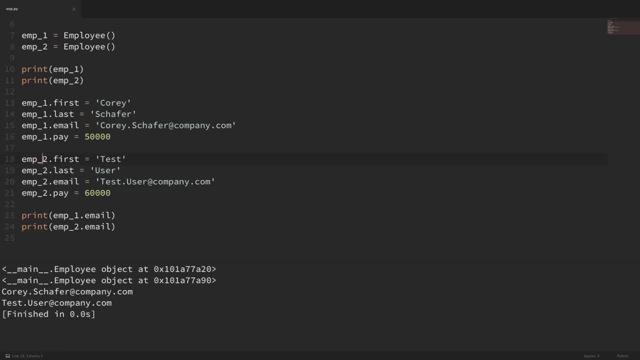 set all of these variables manually. So we're going to set all of these variables manually. So we're going to do this. And it's also prone to mistakes, just like I did whenever I forgot to change the to employee two, So we don't get much benefit of. 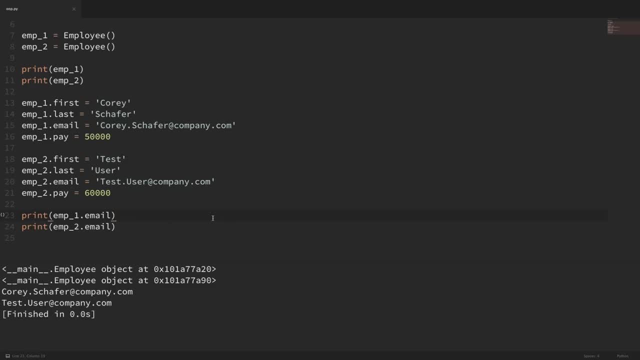 using classes. if we did it this way, So to make these set up automatically when we create the employee, we're going to use a special init method. So now, inside of our employee class, I'm going to create this special init method. Now you can think of this method as initialized. 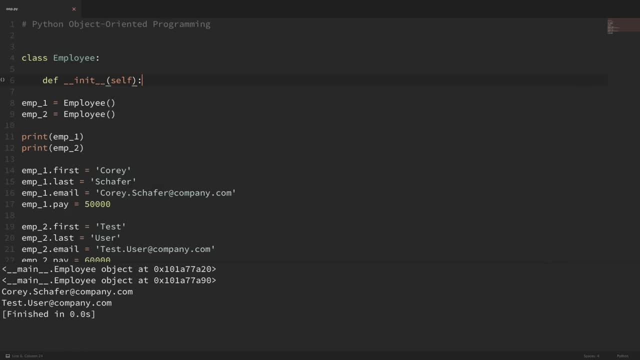 And if you're coming from another language, then you can think of this as initialized, And if you're coming from another language, then you can think of this as initialized as the constructor. Now, when we create methods within a class, they receive the instance as the. 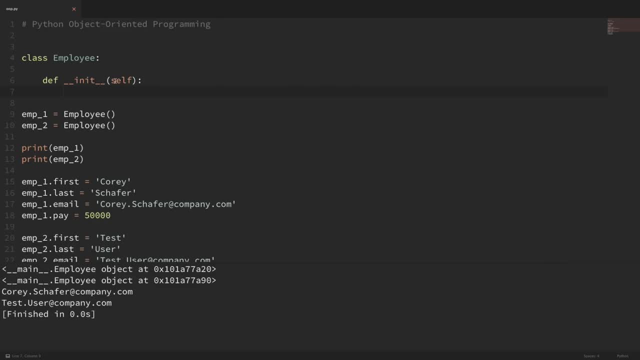 first argument: automatically And by convention we should call the instance self. Now you can call it whatever you want, But it's a good idea to stick to convention here and just use self. So after self we can specify what other arguments that we want to accept. So let's go ahead and 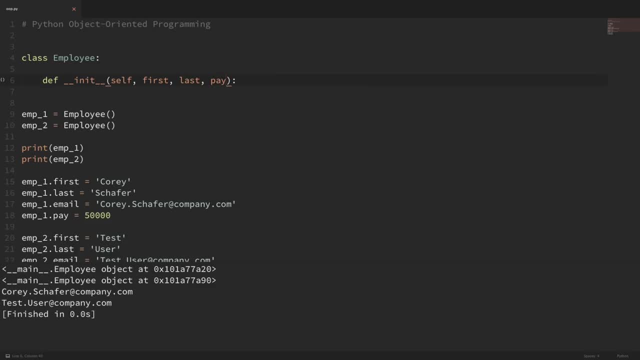 accept the first name, the last name and the pay. And I know that we had email too, but we can create the email using the first name and the last name. So now, within our init method, we're going to set all of these instance variables. So let's do selffirst equals first. And now I'm just going. 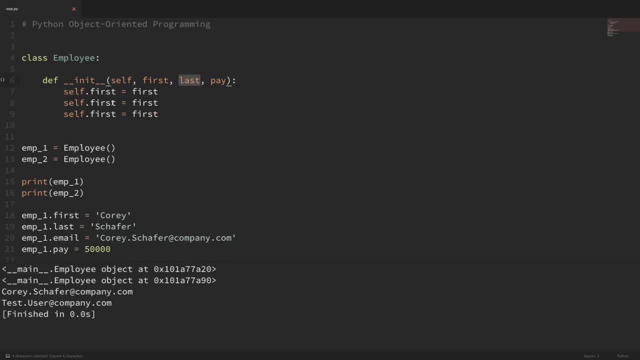 to do this for the rest of them as well. So I'm going to do selfpay or selflast and selfpay, And for the email I can do selfemail equals first plus, and then we'll put a dot between those and then last, And then we'll add on to the end at companycom. Okay, so whenever I 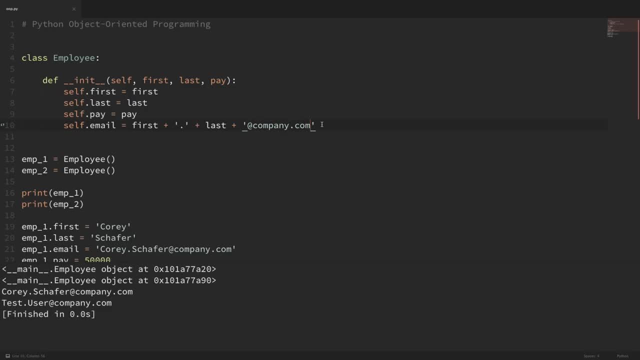 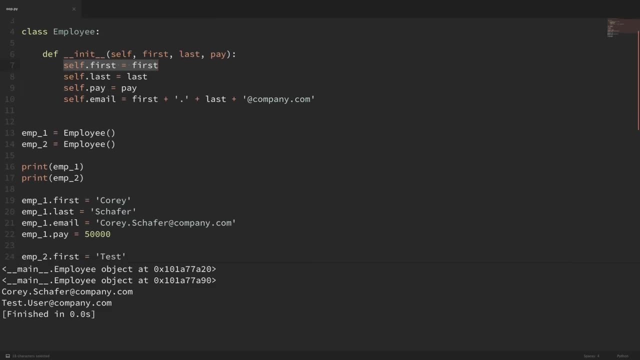 say that self is the instance. what I mean by that is that when we set selffirst equals to first, here it's going to be the same thing as us saying down here that employee1.first equals Corey. Except now, instead of doing this manually, it'll be done automatically when we create our employee. 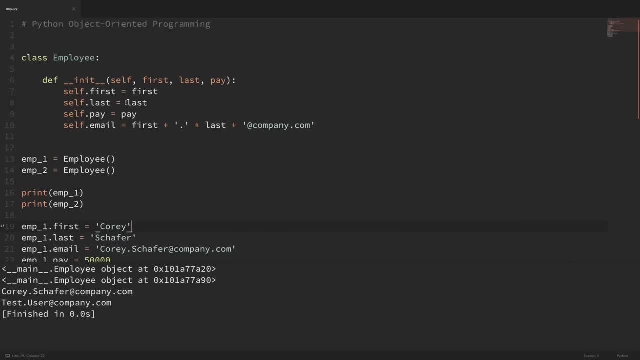 class. Now, these don't need to be the same as our arguments. So, for example, I could make this selffname equals first, but I usually like to keep these similar if possible, So I'm going to go ahead and set that back to selffirst equals first. Okay, so now when we create our instances. 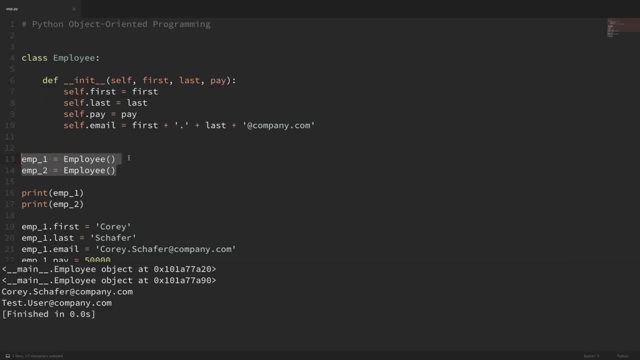 of our employee class right here now we can pass in the values that we specified in our init method. Now our init method takes the instance which we called self and the first name, last name and pay as arguments. But when we create our employee down here, 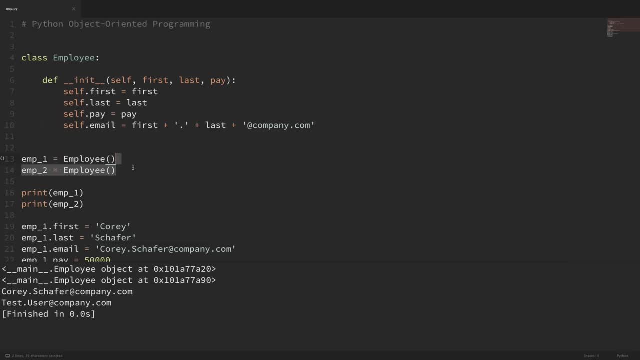 the instance is passed automatically, so we can leave off self. We only need to provide the names and the pay. So we could create these by passing in first, and we have to do this in order. So I will pass in all of the same information that we did manually down there. And for the second one, 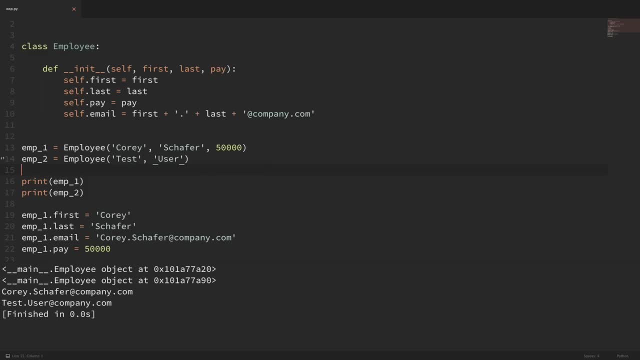 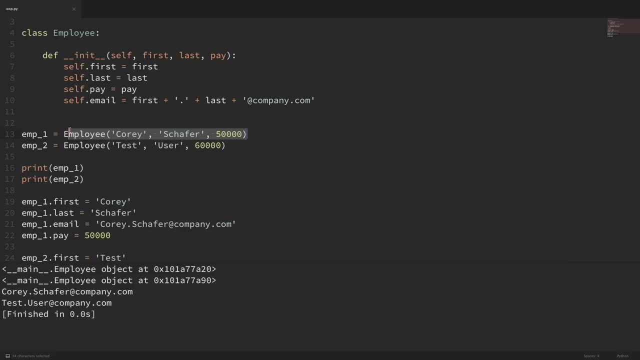 I'll do test and user, And I think I had that at 60,000.. Okay, so what would happen on this line when we create this employee? the init method will be run automatically, So employee1 will be passed in as self. 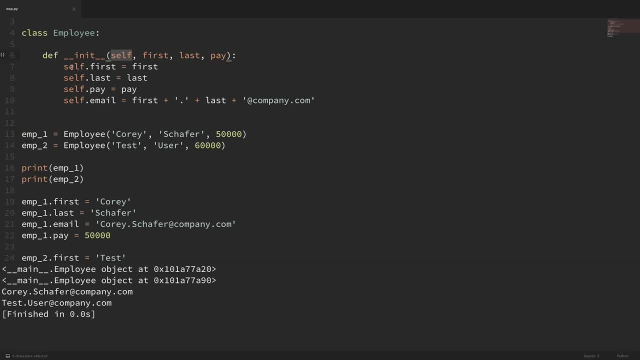 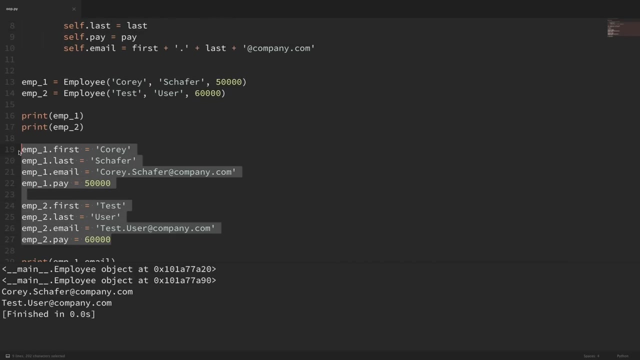 and then it will set all of these attributes. So it'll set: employee1.first is equal to first, which we passed in as Cori, Employee1.last equals what we passed in as last, and so on. So now that we have that init method in place, we can go ahead and delete these manual assignments that. 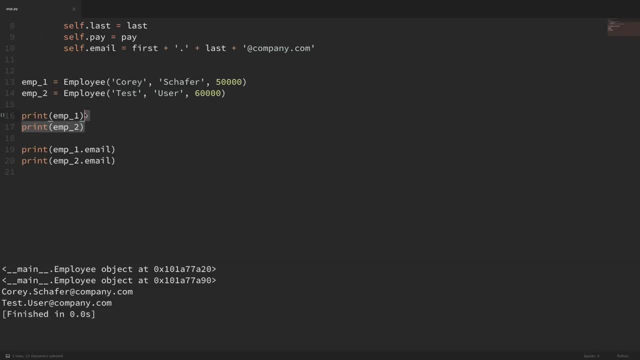 we made down here And you can see by deleting that that we got rid of a lot of code. So I'm going to go ahead and comment out those lines where we're printing the employees And I'm just going to go ahead and print out the email. So if I run that then you can see that that still. 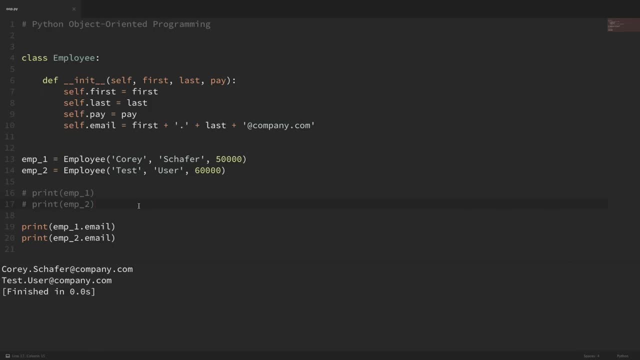 works Okay. so everything that we have so far, like the names and email and the pay, are all attributes of our class. Now let's say that we wanted the ability to perform some kind of action. Now, to do that, we can add some methods to our class. So let's say that I wanted. 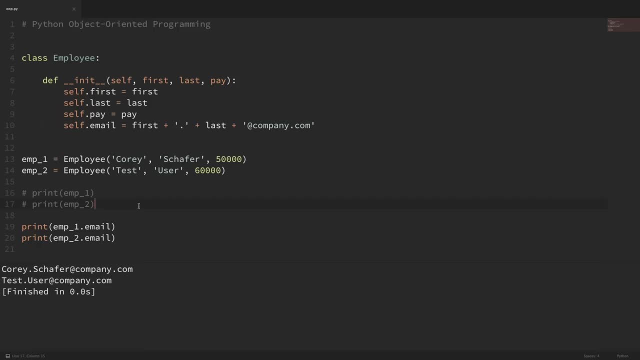 the ability to display the full name of an employee. Now, this is an action that you'd likely need to do a lot with a class like this, So we can do this manually outside the class. if I was to come down here and do print and I could get the full name just by putting in. 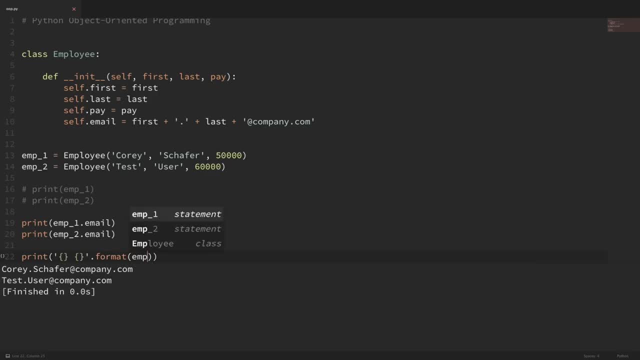 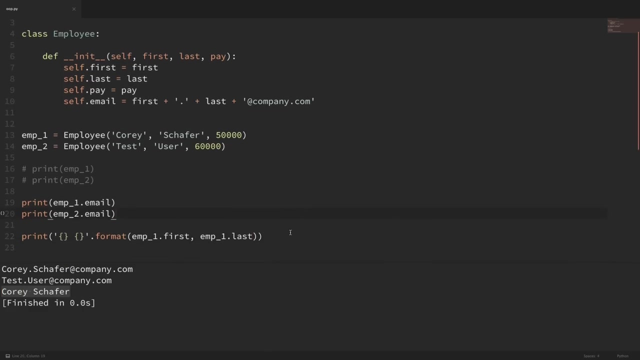 two placeholders there and doing a format and saying employee1.first and employee1.last, And if I go ahead and print this out, then you can see that we got the full name there. But that's a lot to type in each time that you want to display the employee's full name. 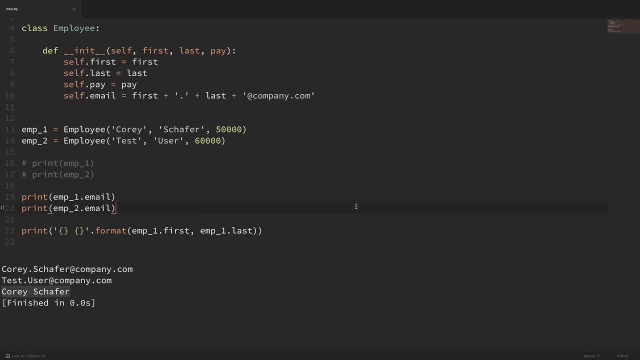 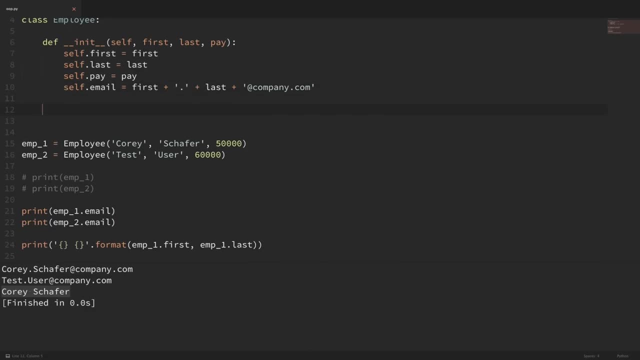 So instead let's create a method within our class that allows us to put this functionality in one place. So within our class here I'm going to create a method called full name, And we can do that with just doing a def of employee1.last. And if I go ahead and print this out, then you can. 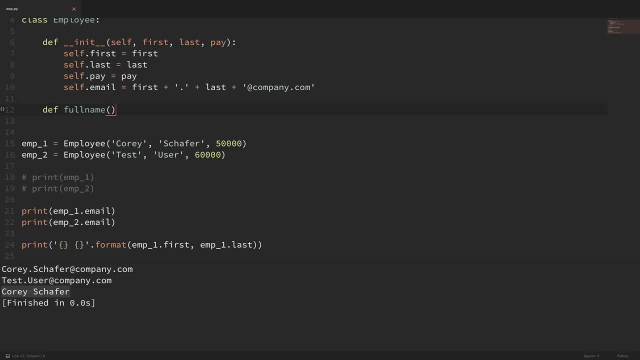 see that we've got the full name. Now, like I said before, each method within a class automatically takes the instance as the first argument, And we're going to always call that self, And the instance is the only argument that we'll need in order to get the full name. So, within this method, 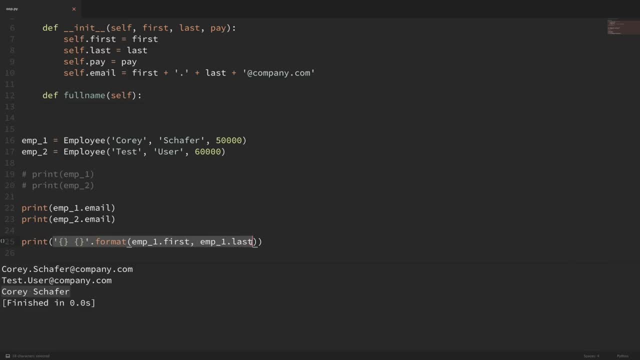 here. I'm just going to take the same logic that we had down here and cut that out, And I'm just going to go ahead and return that. But we have to be careful here, because now, instead of printing employee1.firstName and lastName, I'm going to use self, so that it will work with all. 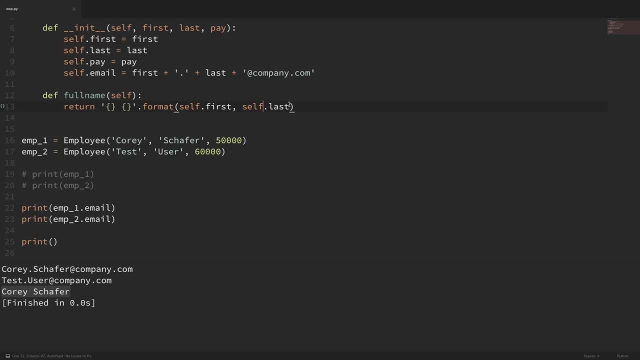 instances. So I'm going to do selffirst and selflast. So now that we created that method, instead of printing like we did before now, I can just come down here and do employee1.fullName and print that out And if I run that then you can see that we got the same thing And notice. 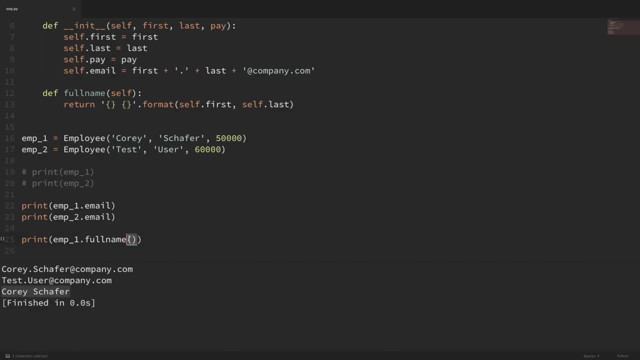 that we need the parentheses here because this is a full name And if I run that then you can see that we have a method instead of an attribute. So if I left the parentheses off and printed this, then you can see that it prints the method instead of the return value of the method. So 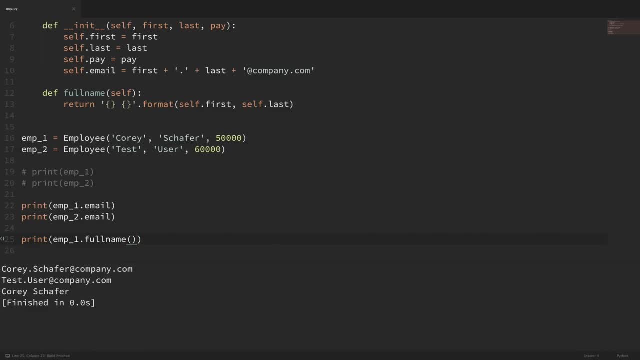 we're going to have to put those parentheses on in order to run that properly. So now we have full advantage of code reuse here. So instead of typing this out for each full name that I want to print now, I can just use that method. So now, if I wanted to print employee2's full name, it's just. 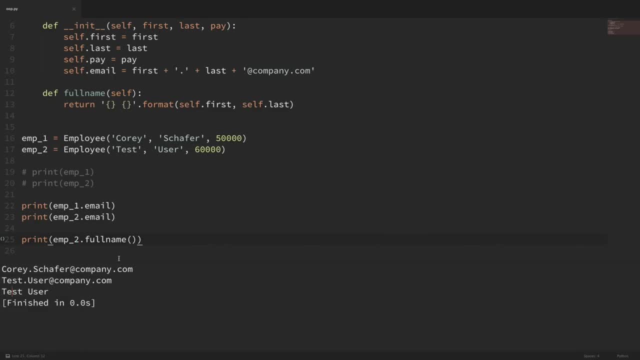 with employee2 and running that and we get the correct answer. Okay, and one more quick thing that I wanted to point out here Now. one common mistake that I see when creating methods is forgetting the self argument, for the instance. So let's take a quick look at what that would look. 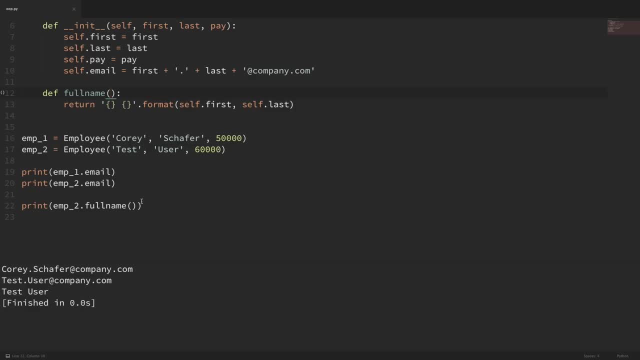 like if we left that off. So now, before I run this, if I just commented out this printing of full name down here and ran this, then you can see I'm actually going to remove these print here as well. Now you can see that this runs without any errors, but if I was to try to run, 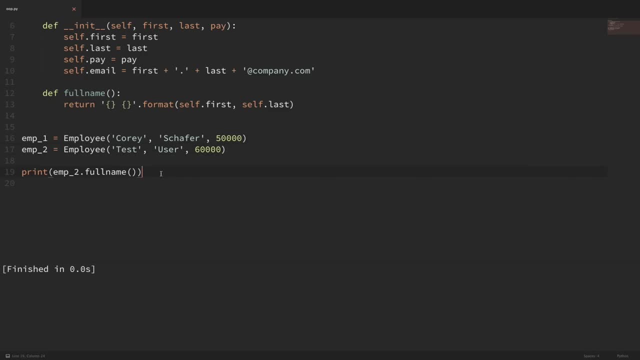 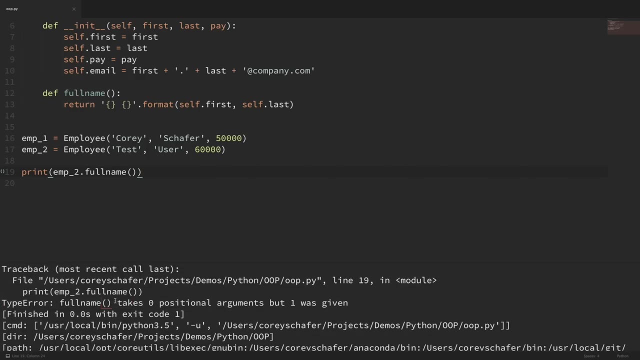 this method that we accidentally left self off of. then run this, then you can see that we get an error. And the error that we got was a type error. full name takes zero positional arguments, but one was given. Now this can be confusing because it doesn't look like we're passing any. 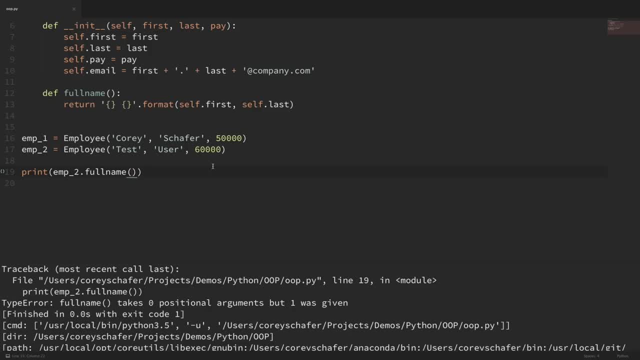 arguments here into full name. but the instance- which in this case is employee2, is going to be the instance that we're passing into full name. So now, if I run this method it's getting passed automatically, So we have to expect that instance argument in our method. 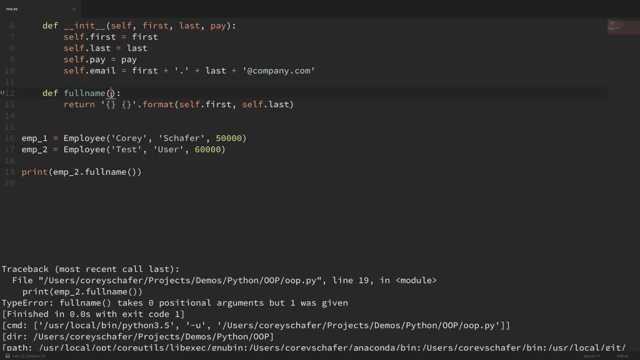 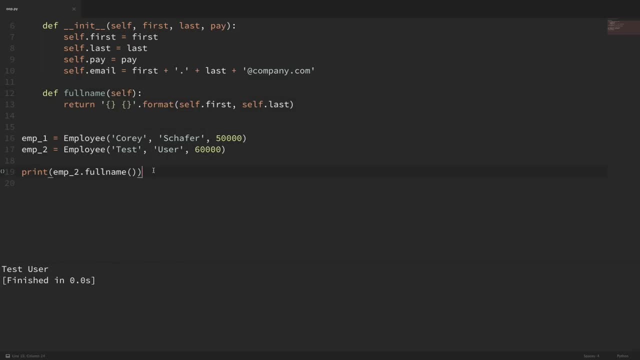 and that's why we added self. So I'm going to come back up here to full name and put self back in and now, running this, you can see that it runs correctly. Now we can also run these methods using the class name itself, which makes it a bit more obvious of what's going on in the 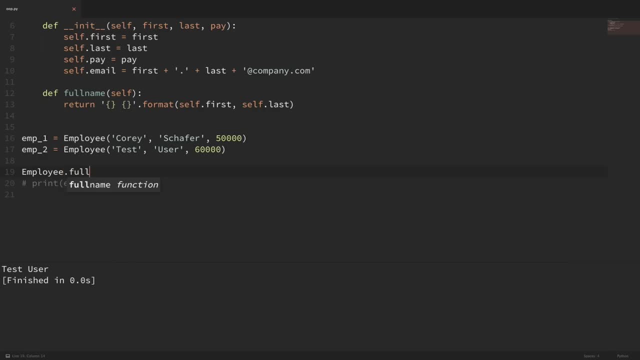 background, Because whenever we do that, so I'll do employee Full name. Now, when we run it from the class, we have to manually pass in the instance as an argument. So in this case I'll pass in employee1.. So you can see how these are similar, but not. 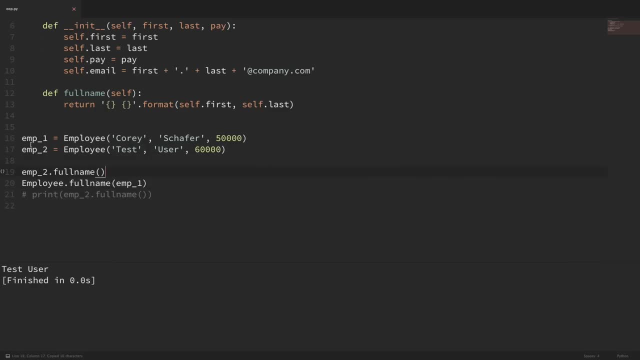 exactly the same. So I'm going to put these side by side just so that we can compare them here. So these two lines here do the exact same thing, But here, when I do employee1, which is an instance and I call the method, I don't need to pass in self, It does it. 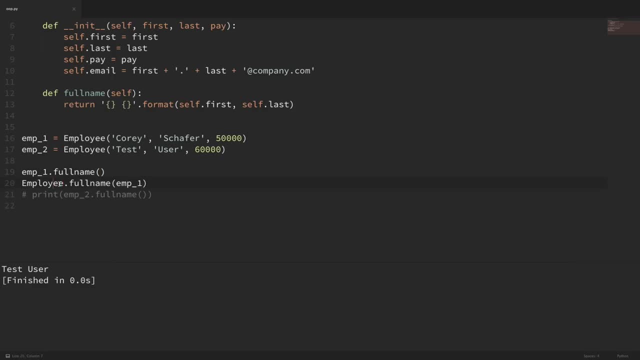 automatically. And when we call the method on the class then it doesn't know what instance that we want to run that method with. So we do have to pass in the instance and that gets passed in as self. And if I go ahead and print this out and run it, then you can see that it works just like. 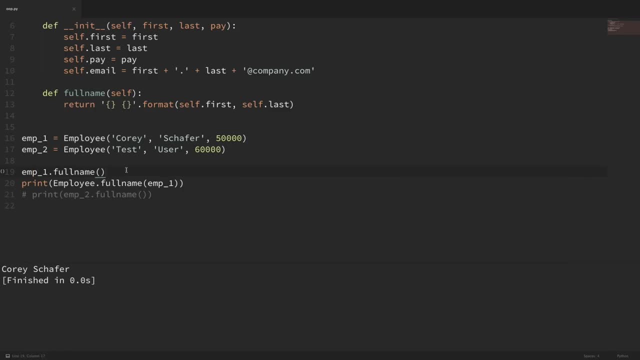 if we were to print out the employee1.fullname- And I wanted to show you that, because that's actually what's going on in the background. when we run employee1.fullname, It gets transformed into this here- employeefullname- and passes in employee1 as self, And that's why we have self.